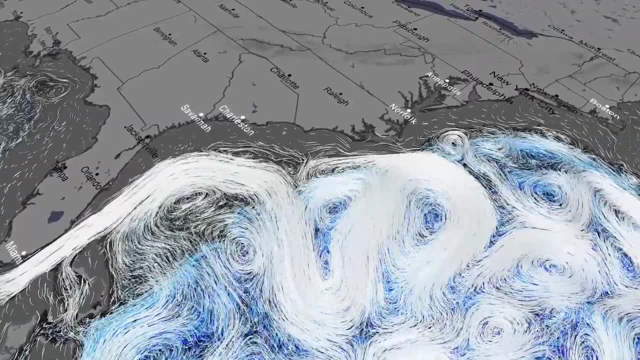 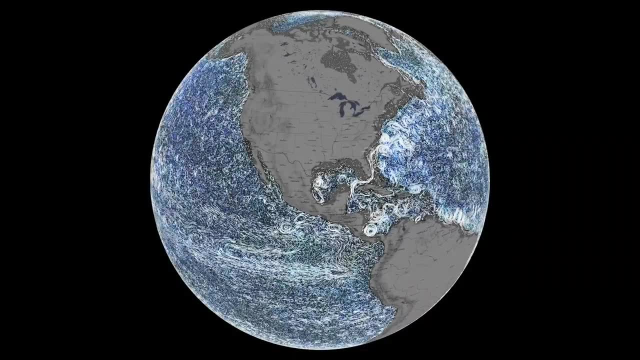 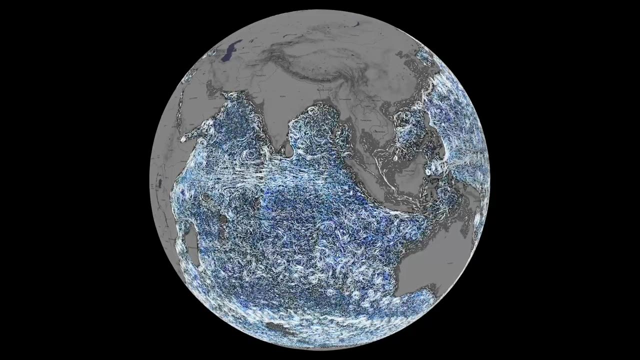 And it also makes it easier to work collaboratively within not only your group but other groups within your discipline, because now everyone's working along the same lines, Principles and guidelines of code. So now more time can be developed on the actual analysis and answering your science questions. 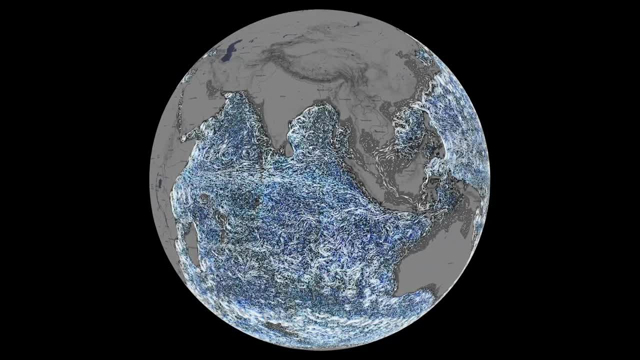 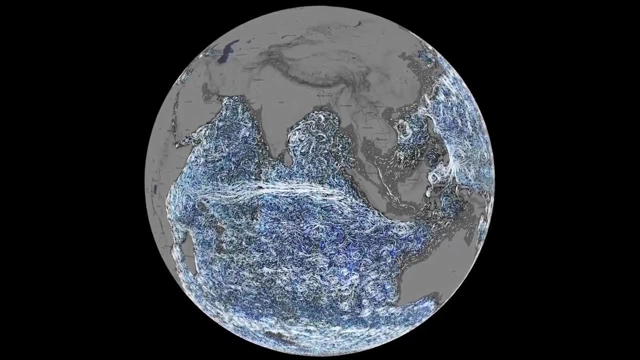 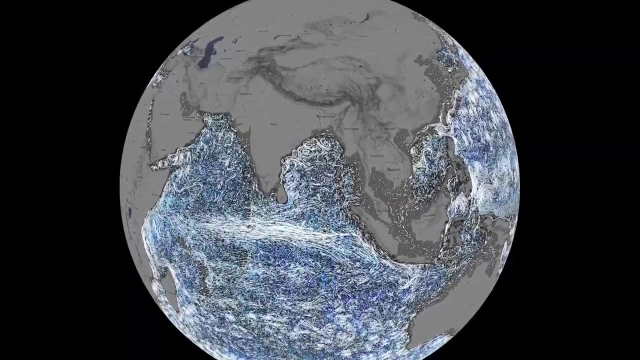 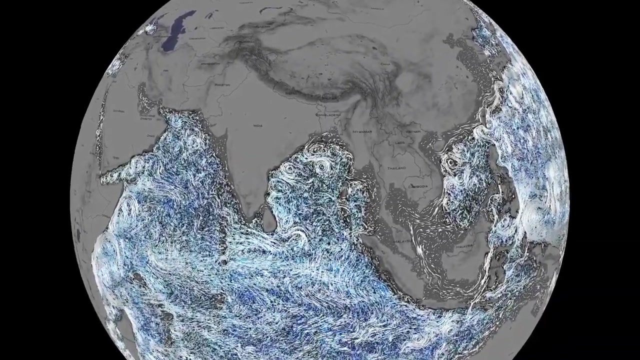 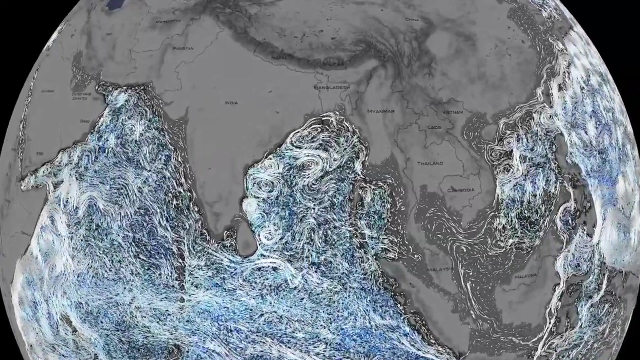 A good example of one of the programs within the physical oceanography program at NASA is ECHO, which is the Estimating the Circulation and Climate of the Ocean Data Assimilation Model. It has created several Jupyter notebooks that help to scientists understand the data formats and read the data and do basic analysis to help integrate it into their science workflows. 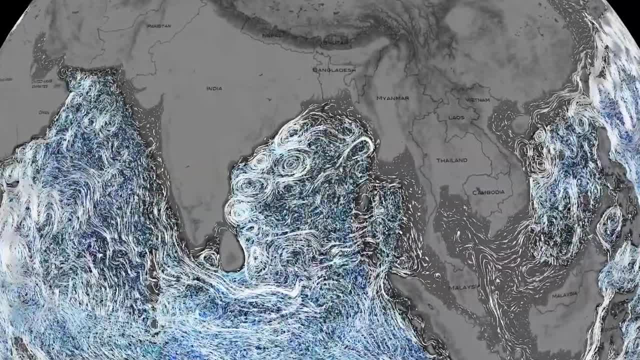 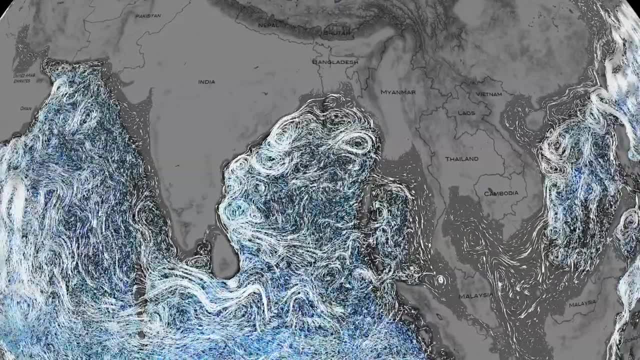 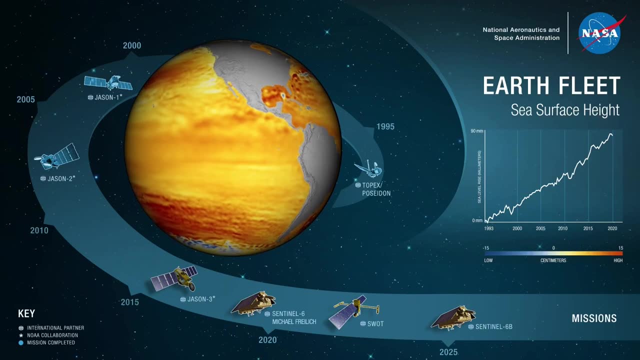 And the success of this is shown by having over 100 new publications within a year. All because ECHO has made it easier for the science community to to use their outputs. The fleet of sea surface height altimeter missions are also within the physical oceanography program at NASA. 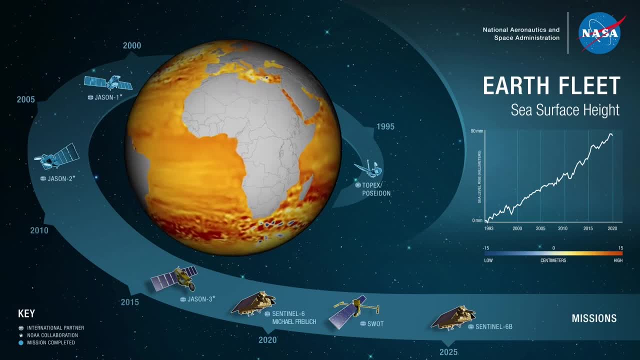 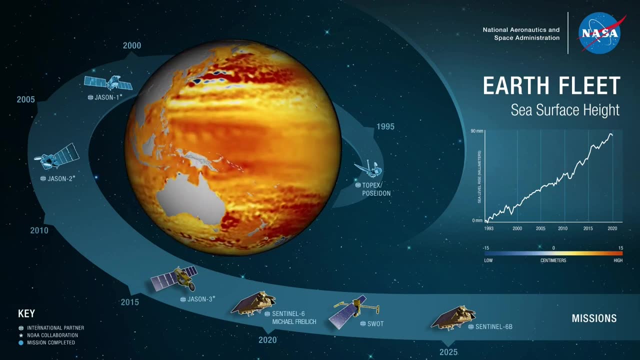 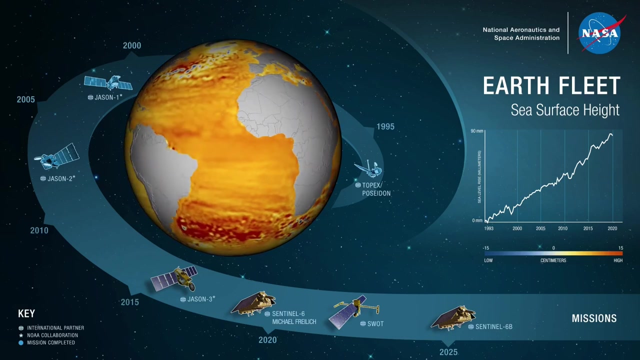 This has started since 1992 with Topex Poseidon and has operated continuously through the Jason series and the recently launched Sentinel-6 Michael Freilich last year in November. And Sentinel-6 is a good example of the continuing progress of open science within the physical oceanography program. 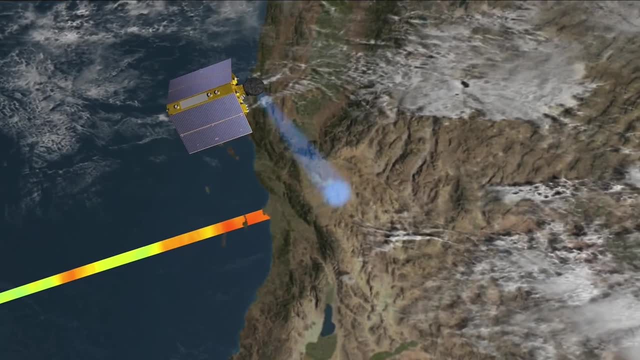 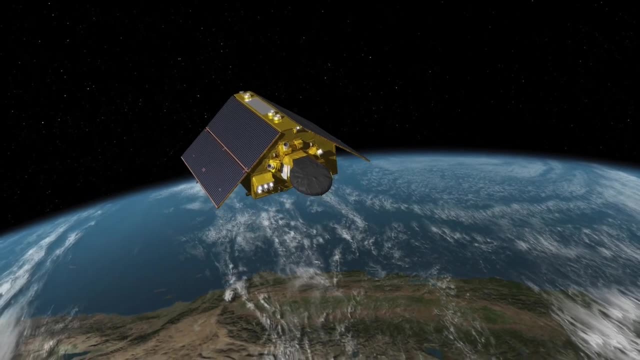 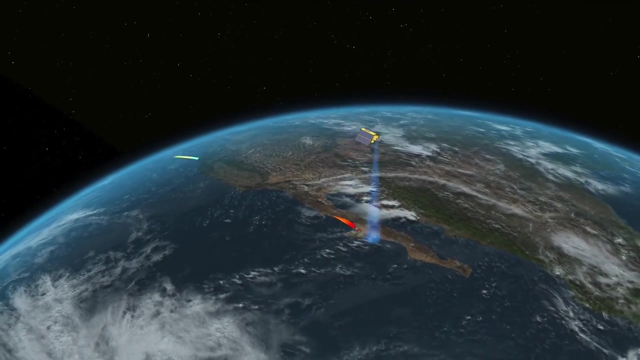 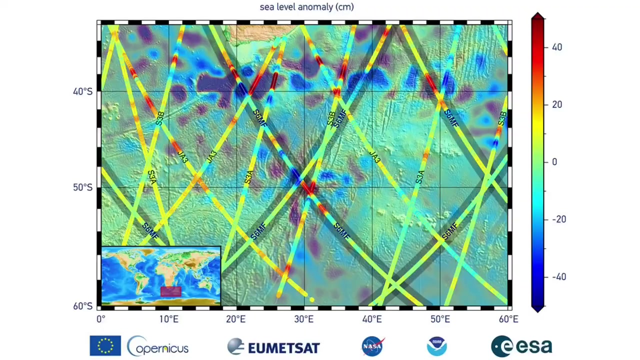 It has continued the tradition of not only measuring sea surface height, but the new tradition of it being the first NASA mission to be fully cloud data distributed. So with this mission and all future altimeter missions from NASA, they will all be found on the cloud. 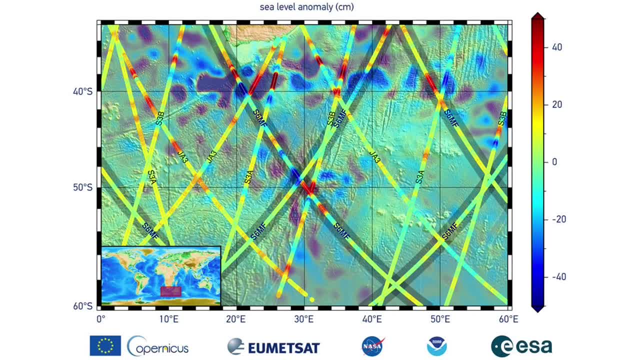 And so, as you can see in this image, this is the current swaths of the operating satellites. Not only is there Sentinel-6, Michael Freilich, but also Jason-3, and then two ESA missions, Sentinel-3A and B. 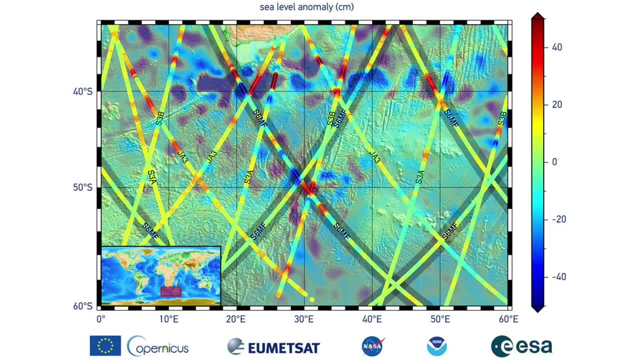 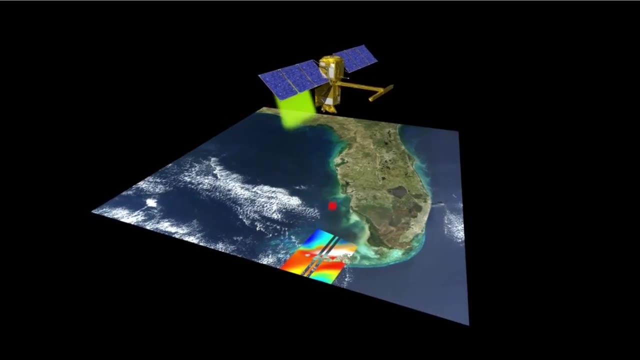 So you can see that there are still gaps within the orbits. So, while the spatial resolution is not very high, you have a very long time series, but not for much longer, Because we are adding in a new mission called SWAT, which is for surface water and ocean topography. 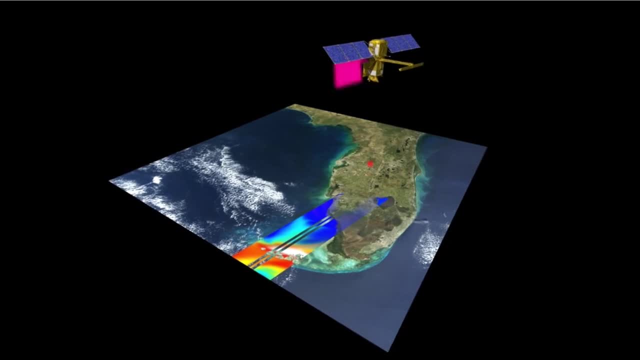 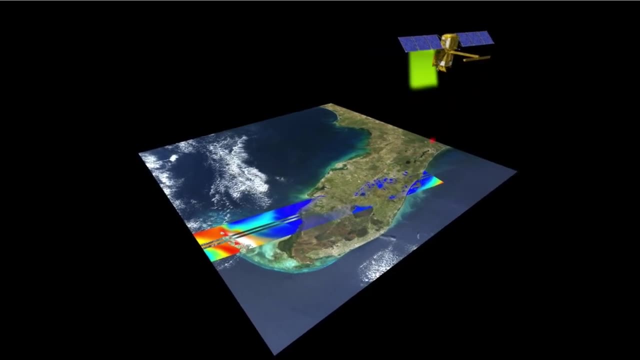 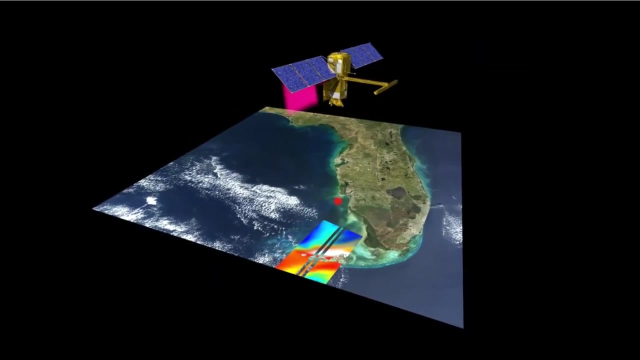 SWAT will be on a different orbit, But not only is it going to be measuring sea surface heights, but also lake and river heights over the surface of land. And the big thing about SWAT is that its data is going to be very large because it is an interferometer. SAR. 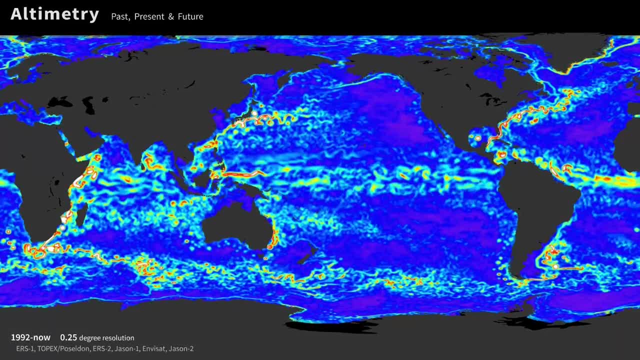 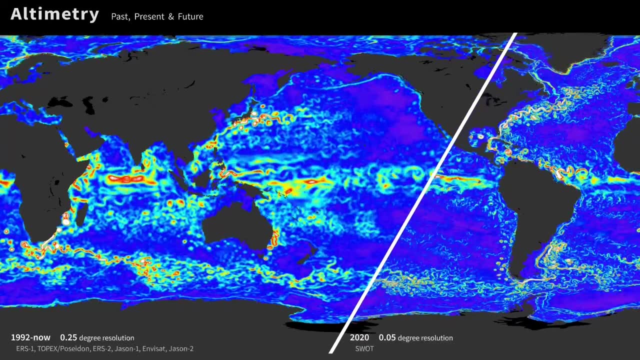 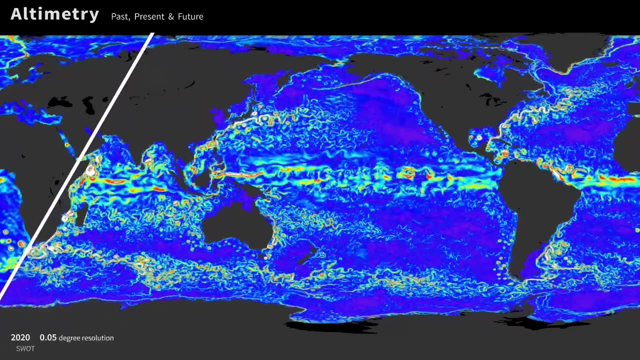 And you can see in this animation of currency, it's derived from altimeters. You can see that this is the current spatial resolution that we have now combining all the satellites together And when SWAT launches in 2022, this is what the expected resolution is going to be from that one mission alone. 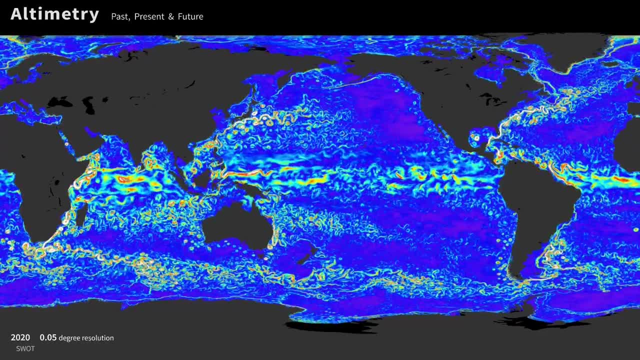 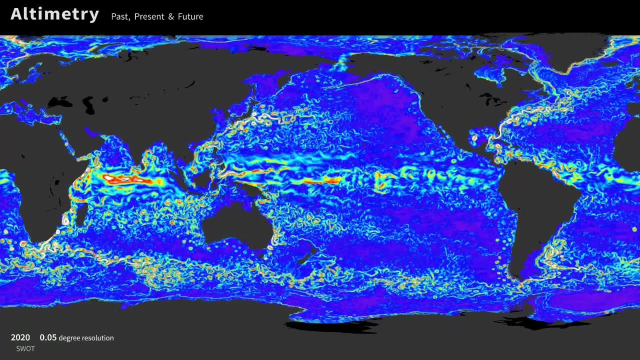 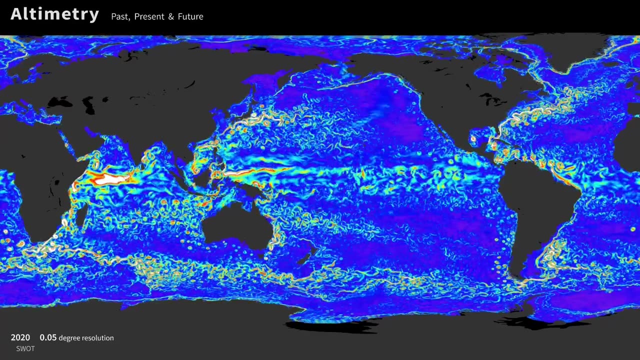 So, even though we will not have a long history of SWAT data, we have very high spatial resolution. So that's why SWAT is also being put on the cloud, because the amount of time it would take for downloading and doing data analysis on that type of volume of data is going to take a very long time. 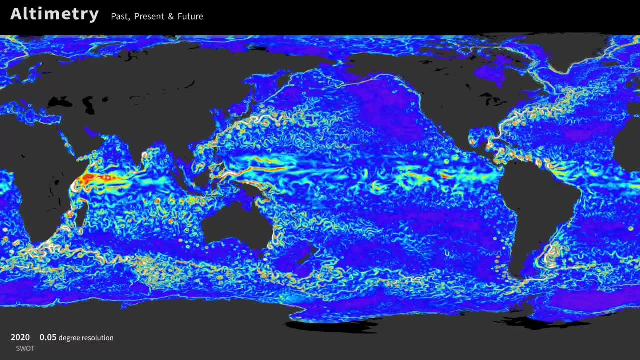 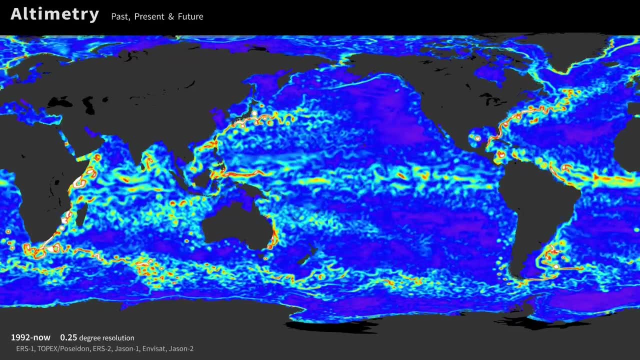 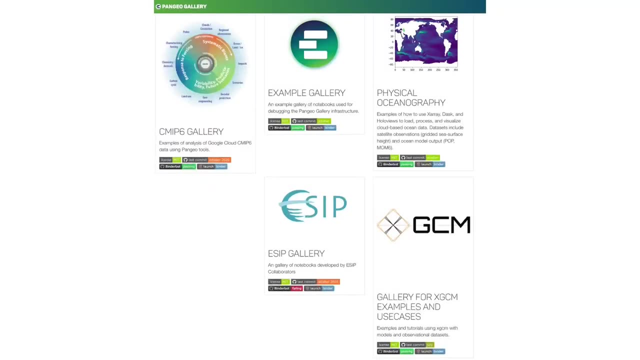 And so being able to put your code next to the data will help improve the amount of time that it takes for you to do your basic analysis as you would do it now if you haven't already switched over to the cloud. Of course, just switching over your workflow into open science does take some effort. 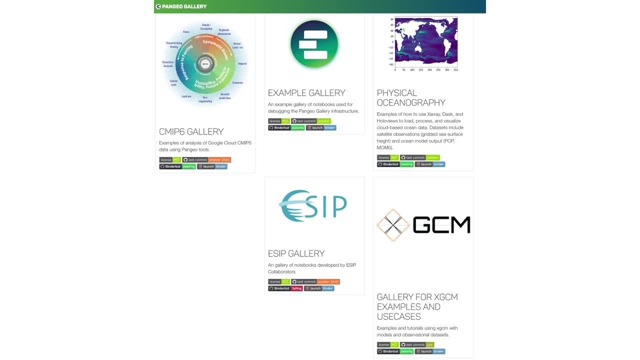 So there is the Pangeo project. It is sponsored by NASA and NSF And it is basically trying to coordinate science and software and compute infrastructure so that it can help promote science that is open, pre-producible and scalable. So these are all Earth scientists who have switched over to open science.